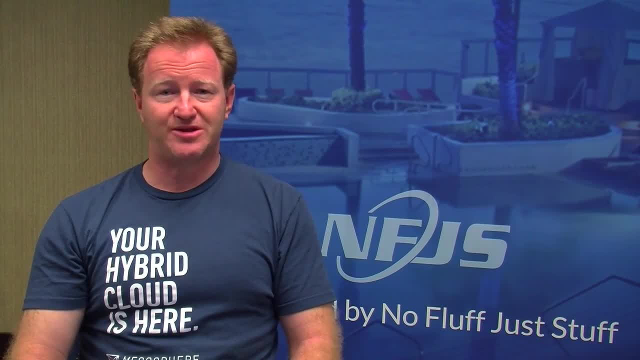 one that's in dmessages, But all of that now is being standardized in an interesting way. So if you're looking at systemd, if you're looking at etcd, if you're looking at the journal- meaning journal patrol- and if all of that is meaningless to you and you don't, 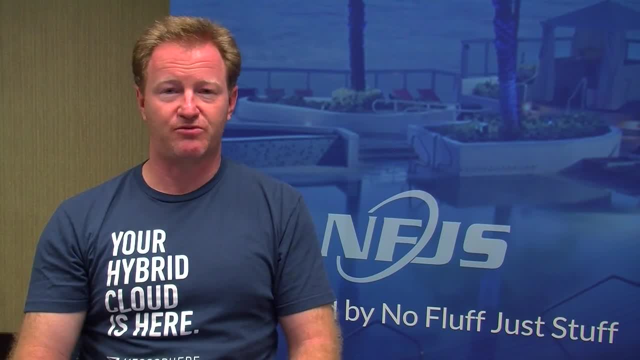 understand it. this is the right talk for you. We're going to go through and understand this new platform. We're going to look at the tooling that's necessary. We'll actually be doing a lot of demonstrations, but the point is to come up to speed quickly on some of these new technologies. or these new platforms. 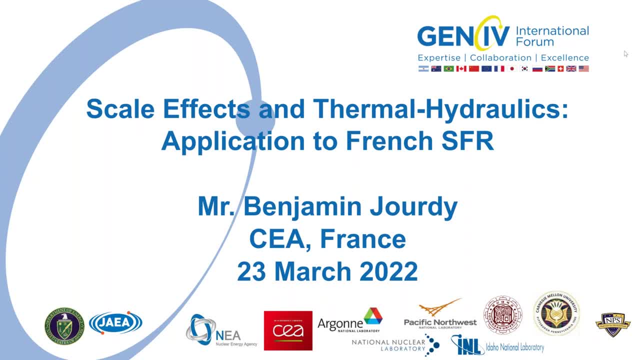 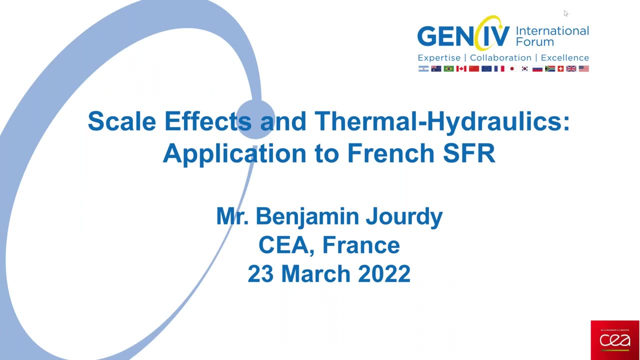 Welcome everyone to the next GEN4 International webinar presentation. Today's presentation on Scale Effects of Thermal Hydraulics: Application to the French SFR will be presented by Mr Benjamin Jordy. During today's introduction is Dr Patricia Pavier. Patricia is the group leader at the Pacific Northwest National Laboratory. She's 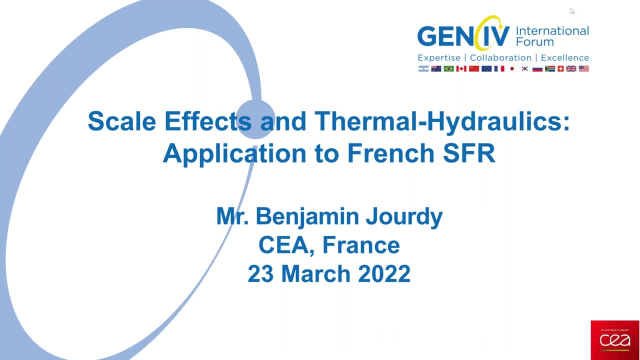 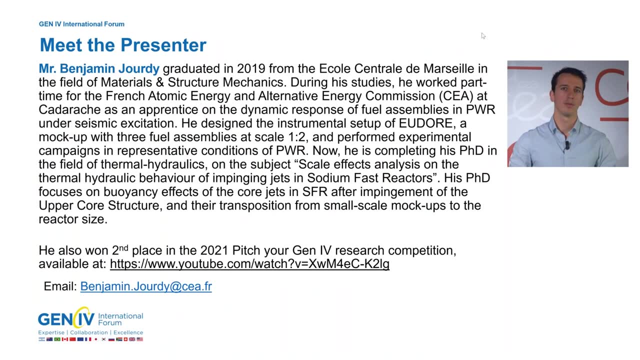 also the co-chair of the GEN4 International Forum Education and Training Working Group. Patricia, I give you the floor. Thank you so much, Bertha. Good morning everyone and good evening. I'm very happy to have Mr Benjamin Jordy with us today. He graduated. 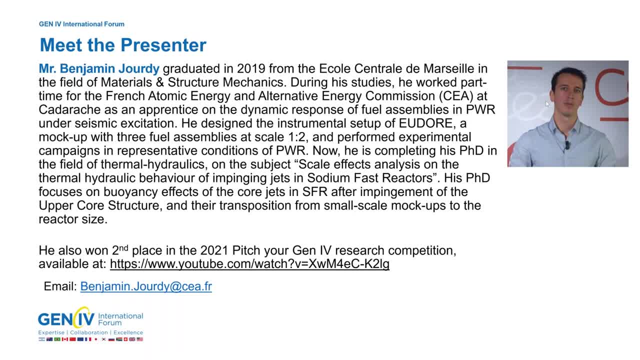 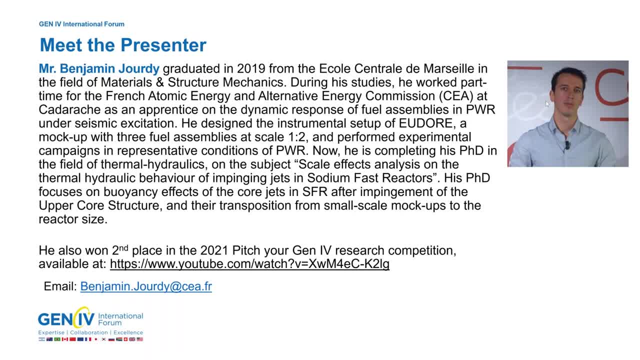 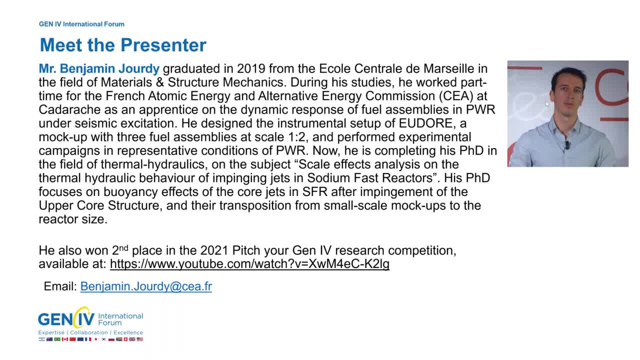